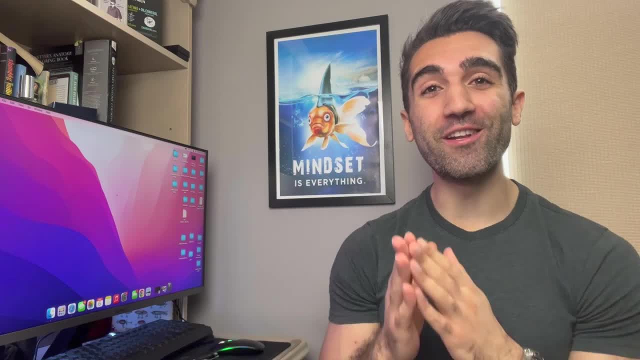 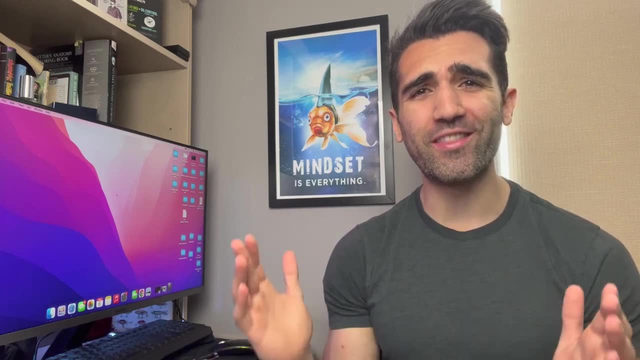 many different reasons to practice medicine in one country or the other, but in today's video I did want to address this topic right here and see if there actually is a big, substantial difference between the two countries and if you're interested in this type of stuff, if you're interested in 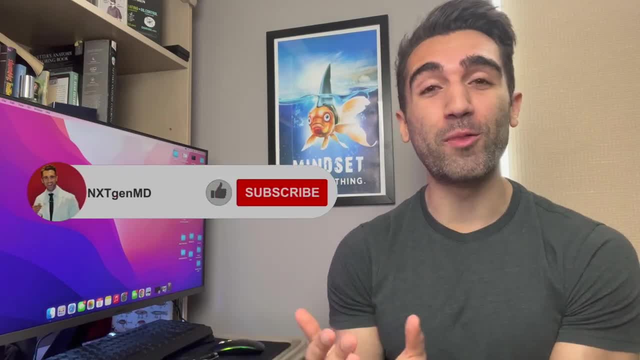 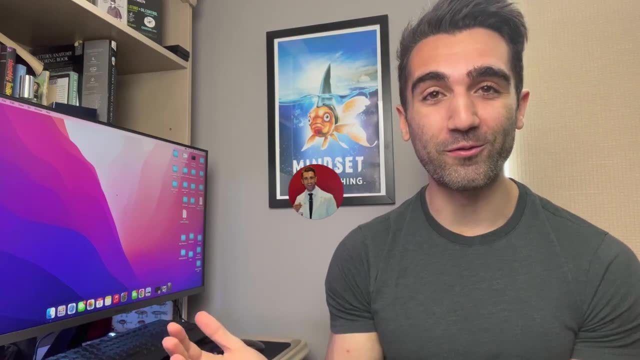 learning a little bit more about medicine. a behind the curtain. look at what the profession is actually like and you want to see more in the future. first of all, leave a like on the video. Second of all, subscribe to the channel And there will be more coming out in the future. 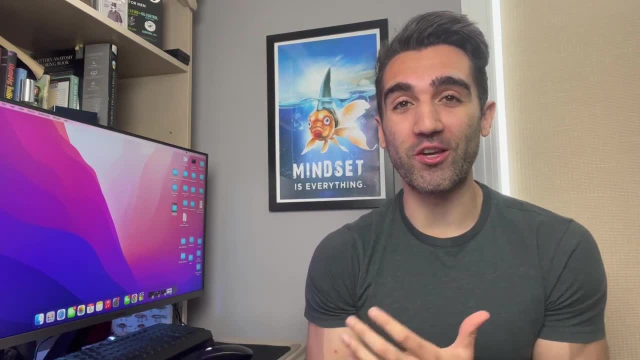 And before the video gets started, I'd love to hear from you guys. Let me know in the comment section below What do you think. Is it better to practice in Canada or the States? Is it because of salaries? Is it because of some other reason? 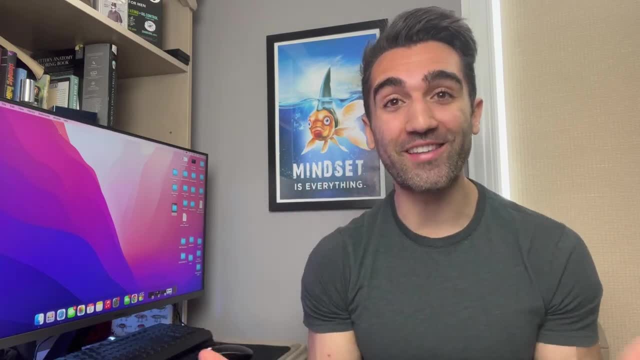 Why would you choose to practice in one place or the other, And what are some questions that we need to ask ourselves when deciding where we want to work? So here's what we're going to do, And this is how we're going to break things down. 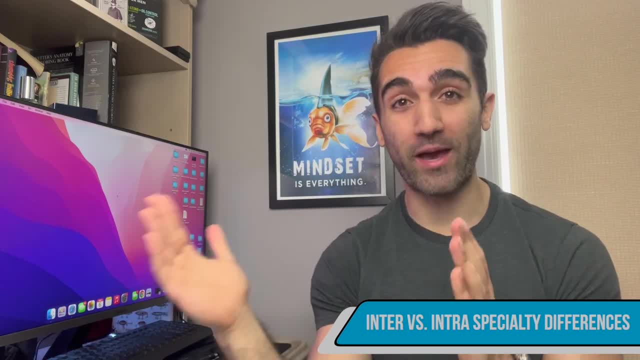 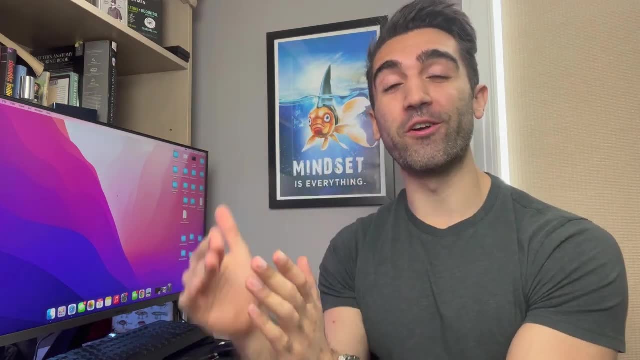 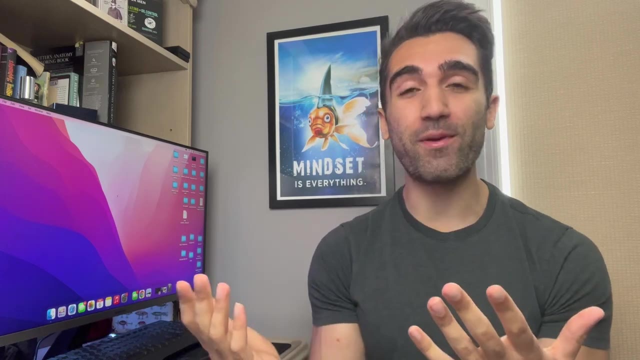 For those of you that don't know, salaries and medicine exist on a spectrum and on that spectrum We have to account for inter specialty variability in salary and then intra Specialty variability in salary. inter specialty variability means that, for example, family medicine doctors on average do not get paid as much as some of these surgical subspecialties. And we have to account for those differences. But on the other hand, intra specialty variability in salary means that even within the profession of family medicine, you will find family doctors get paid three to four times as much as some of their colleagues, even within the exact same specialty. 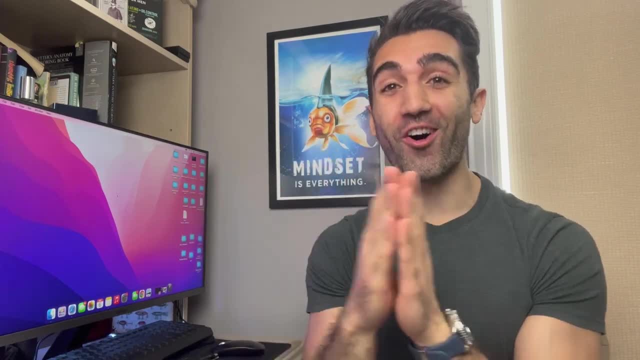 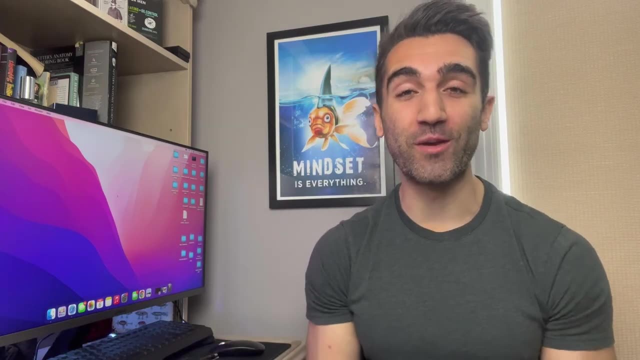 So what we're going to be doing is looking at a few different specialties on the spectrum To see what the differences are and some things that you need to keep in mind If you are going to try and compare how much doctors make from one country to another. Now, on that note, the first specialty that we're going to be looking at is family medicine. This is on the lower end of the spectrum when it comes to pay, But, having said that, it is the specialty that I chose to get into. It was my first choice and it is what I believe to be the best medical specialty to get into. 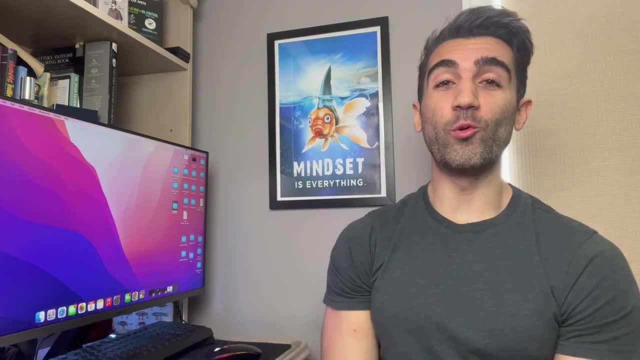 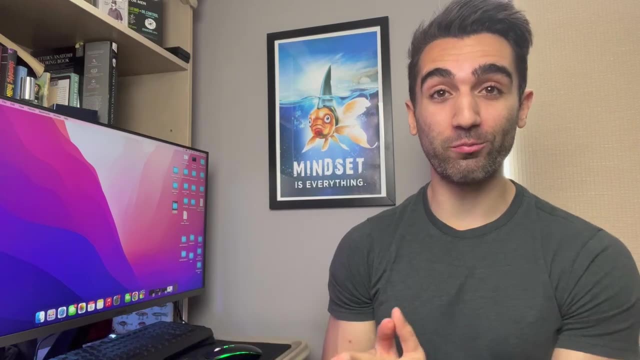 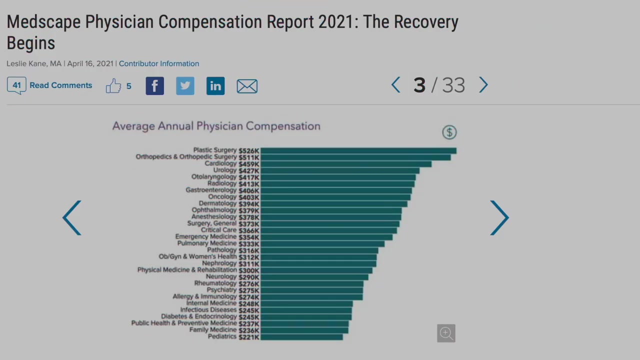 If you are a Canadian physician, but more on that in the future video. when we compare the salary of family medicine doctors in Canada versus the United States, using the most official resources that we could find, those being the CMA specialty profiles for the Canadian doctors and the Medscape 2021 physician salary slash compensation report down in the States. 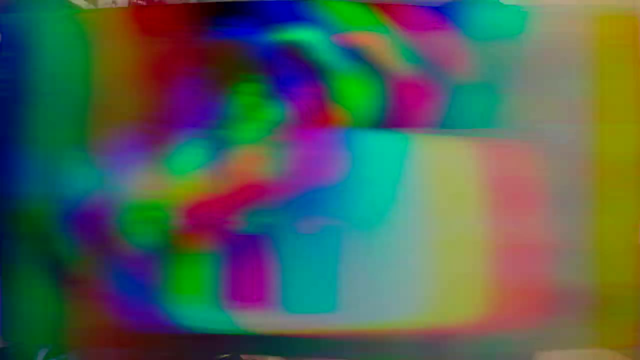 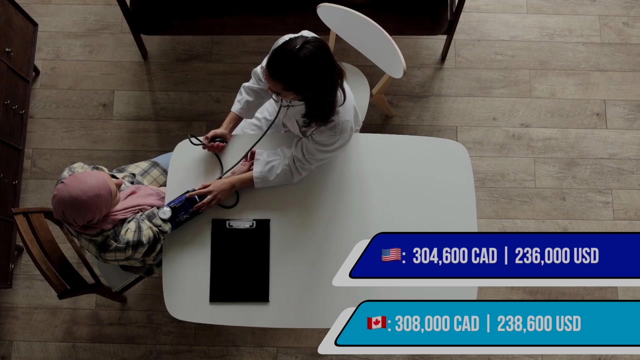 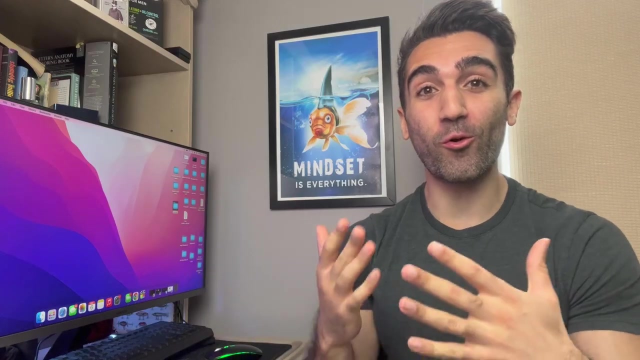 What we see is that the American family doctors will average about $236,000 per year and their Canadian counterparts will be making somewhere around $308,000 per year. Family medicine doctors in Canada, relatively speaking and when compared to their American counterparts, are able to hold their own in terms of salary. And especially in provinces like Ontario, for example, if you have a newly minted family doctor that is willing to do those 50-60 hours per week, pick up some additional shifts. maybe some rural emergency medicine whenever possible, some low-risk obstetrics. 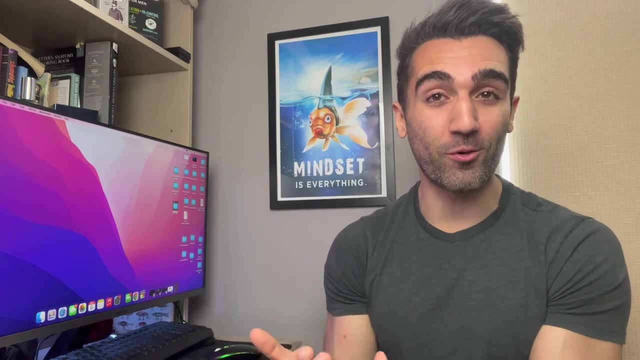 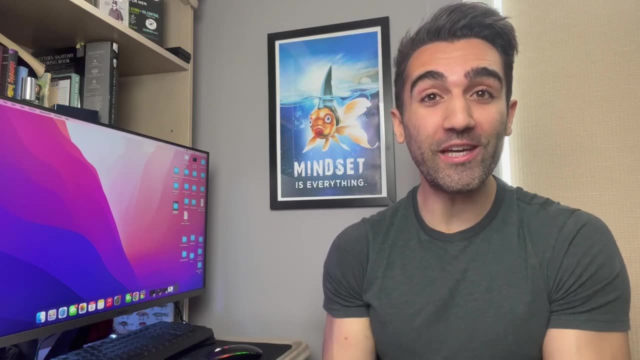 they do have that potential to even surpass the American counterparts when it comes to family medicine, And taking it a step even further than that. I've spoken to many family doctors here in Ontario that have agreed with the statement that they believe that it is. 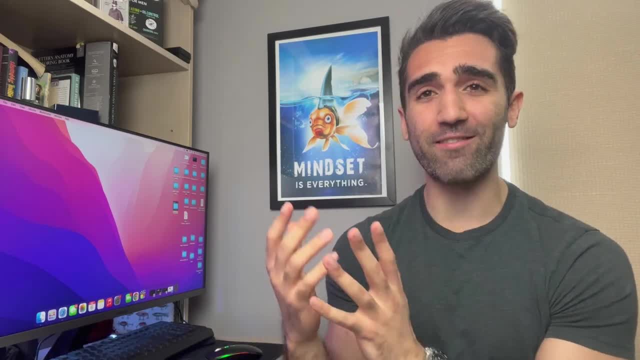 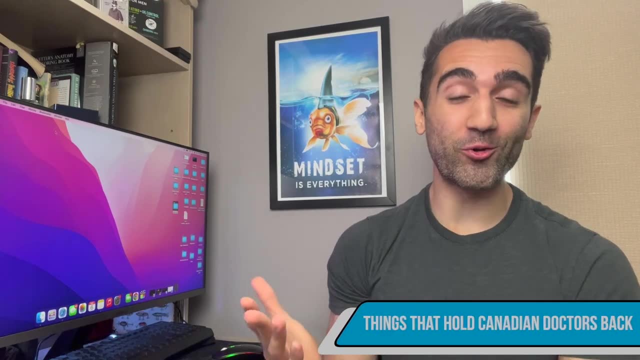 more fiscally responsible, more fiscally advantageous to practice in Ontario than it would be to move down to the States and open up a practice there. But at the same time, let's not get carried away, because there are two very important factors to keep in mind. 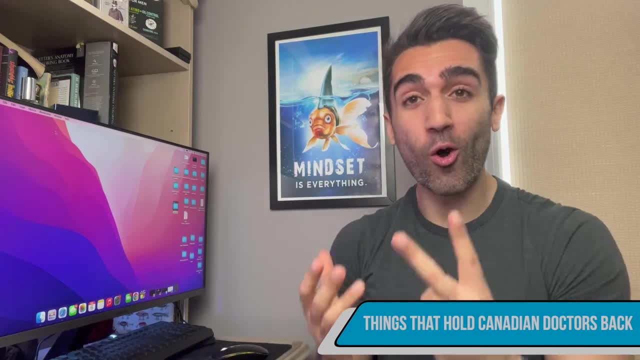 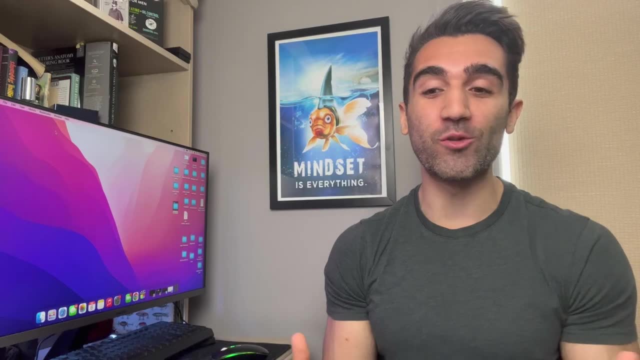 if you are trying to compare the two countries, and it is something that holds back the earning potential of any physician is trying to enter Canada, And I don't think a lot of people have this realization when they're considering the process in the beginning. The first thing that we need to talk about is the conversion rate. 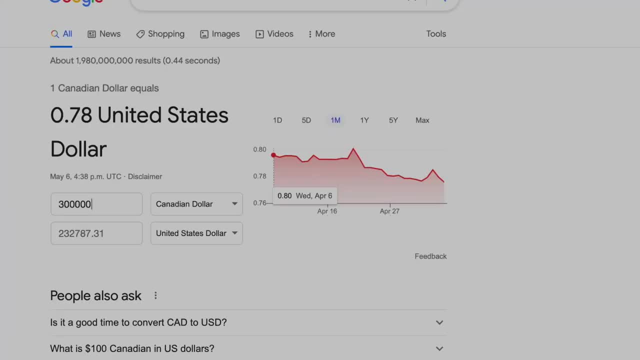 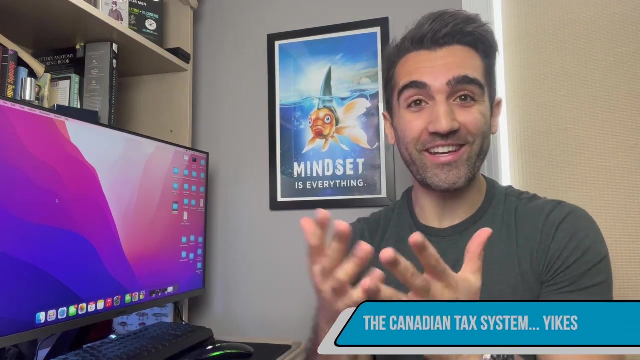 For every $300,000 that someone makes here in Canada, at the current conversion of one Canadian dollar equaling about 78 American cents, you get $300,000 turns into about $230,000 American just from conversion alone. On the second hand, in something that only Canadian individuals could really appreciate, 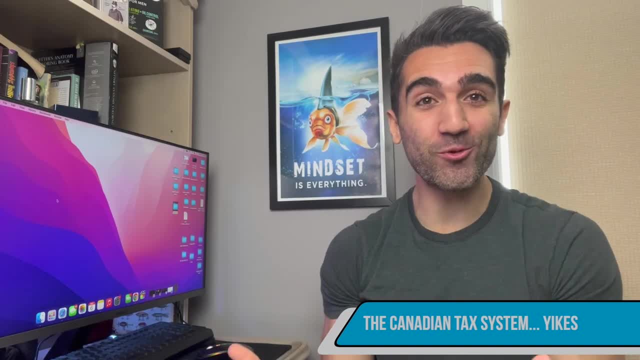 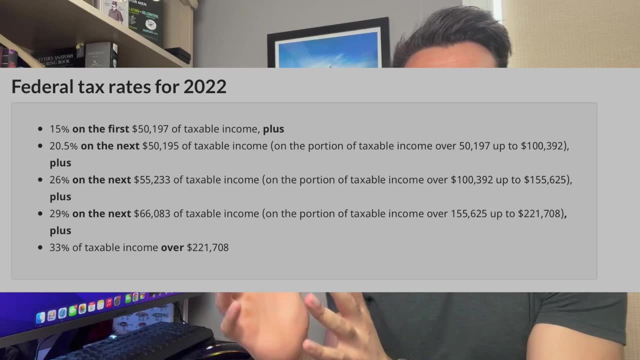 until you've lived through it yourself. obviously is that Canadian individuals- doesn't matter if you're a doctor or not- are paying some of the highest income taxes anywhere in the world, And this becomes particularly noticeable to physicians that have incomes over $200,000. Let's say, in the highest tax bracket, which many physicians will be, you're getting charged upwards of 33% income tax on everything over that $220,000 mark, which is crazy, especially when compared to some of these southern states, for example, like Florida, that I'm pretty sure still don't have state-level tax. 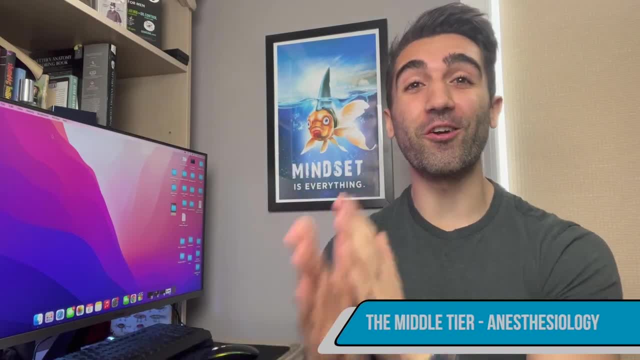 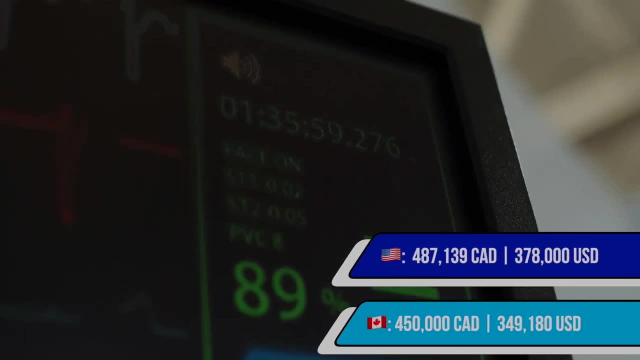 Now the second section of the spectrum that we are going to be looking at next are the middle-tier earning specialties, And for this one we're going to be comparing anesthesiology. Canadian anesthesiologists report making on average about $450,000 Canadian dollars. 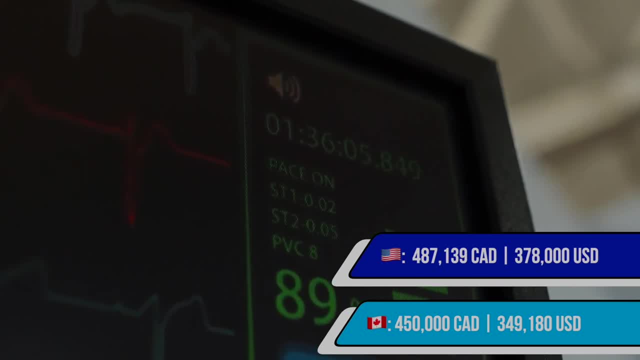 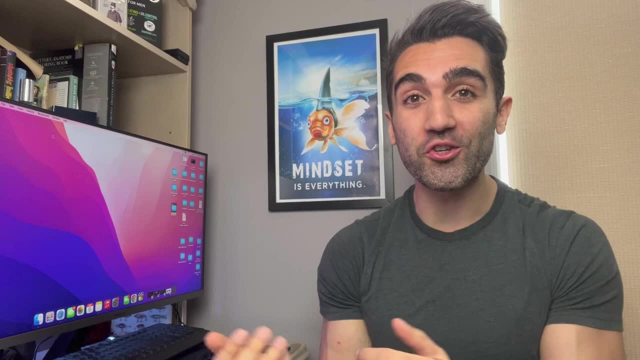 whereas in the United States they report making somewhere around $378,000 American dollars. Now what you'll see here, even in the middle tier, is that at first glance, even after the currency conversion, it looks as though the specialists in the different countries seem to be making approximately the same amount of money. 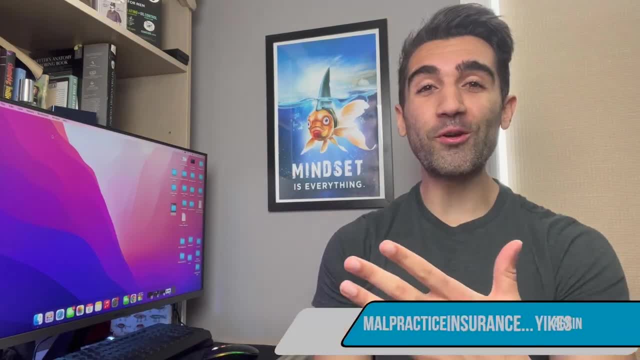 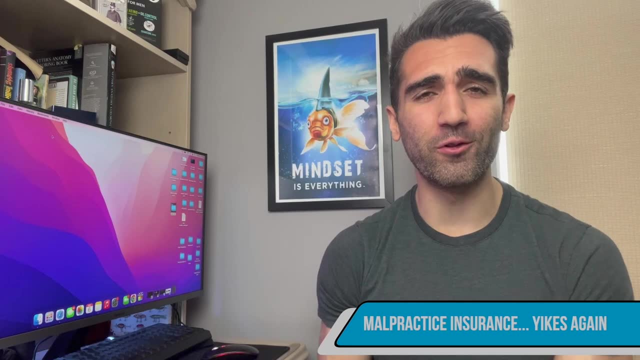 And we'll just set those pesky taxes aside for a second. But this is where you need to take into account even another factor that a lot of people, myself included, didn't consider, until you actually start looking at paying off student loans and things like that. 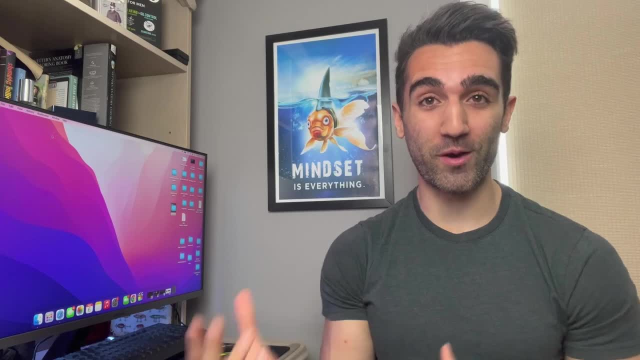 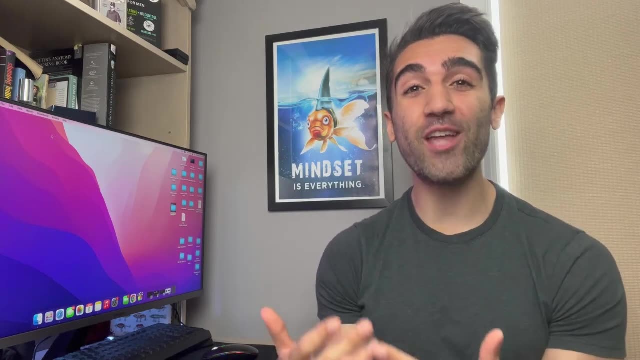 is the concept of malpractice insurance And in speaking with different specialists from here from down in the States, it seems like the cost of malpractice insurance varies by both your specialty and where you are practicing, And the general consensus seems to be that malpractice insurance down in the United States tends to be a lot more expensive than it is here in Canada. What I would recommend to anyone deciding whether or not they want to go and practice in the States or Canada is to look into how much some of the additional expenses incurred by your particular profession are going to cost you in the two different countries. 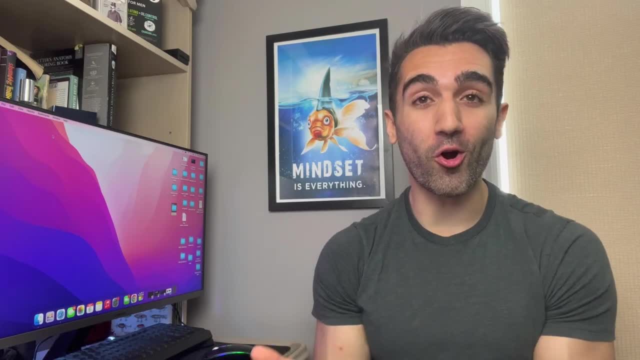 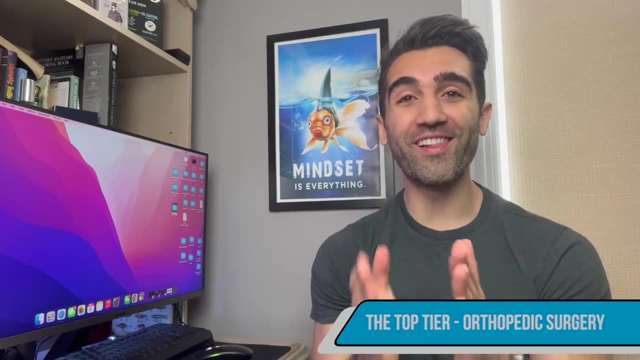 It is not a stretch to say that, depending on what province you're working in, there are some anesthesiologists that here in Canada, could also hold their own compared to the salaries of their American counterparts. Now, finally, the last section that we are going to be looking at is the high end of the spectrum. These are all of the surgical subspecialties. The surgical specialties in general tend to make more than the non-surgical specialties in both systems, But what I found to be crazy is just how much more the surgeons in the States tend to make than the Canadian surgeons here. And in speaking with a few Canadian surgeons that have worked in the States and worked in Canada as well, the general consensus seems to be that you're making a lot more money down in the States for surgery. There are many reasons why that is, But, for example, the Canadian surgeons here 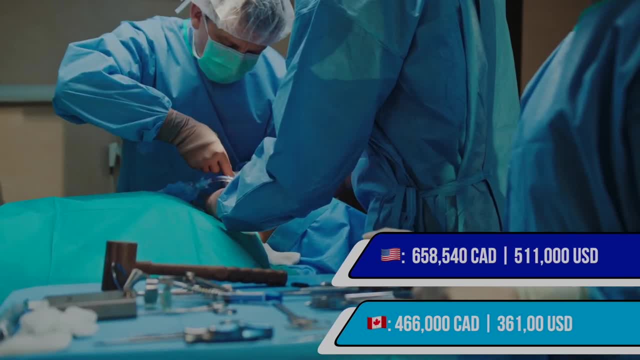 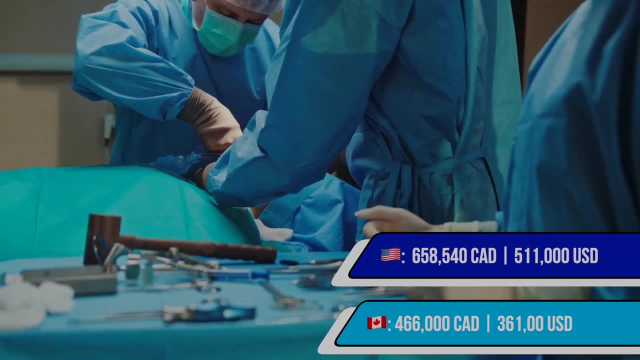 the orthopedic surgeons will report making somewhere around $466,000 per year as an average. This could be higher or lower depending on a few different factors, But in the States the average salary for an orthopedic surgeon across all of the different states is around $511,000 American after the conversion. That is a substantial difference. But when we start looking at the outliers, the top earners in these fields, it seems like orthopedic surgeons and many of the other surgeons that are making millions of dollars down in the States. 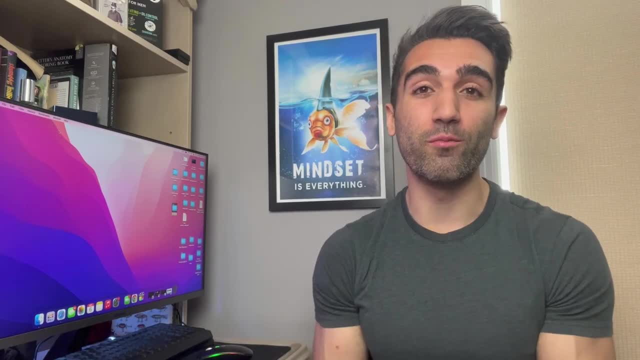 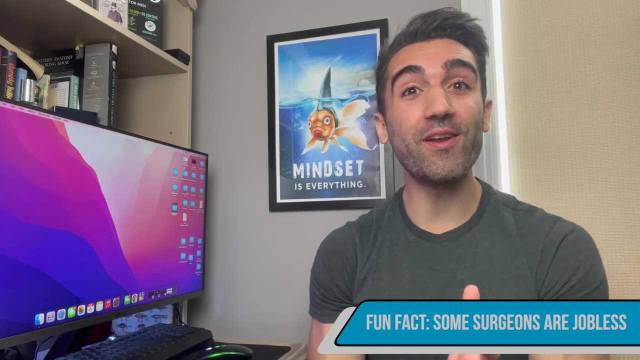 whereas that becomes a lot less common here in Canada. if you are employed in a hospital- And I mean that's if you could even find a job as a surgeon here in Canada. Another little known fact for many people is that there are many areas of surgery here in Canada right now. 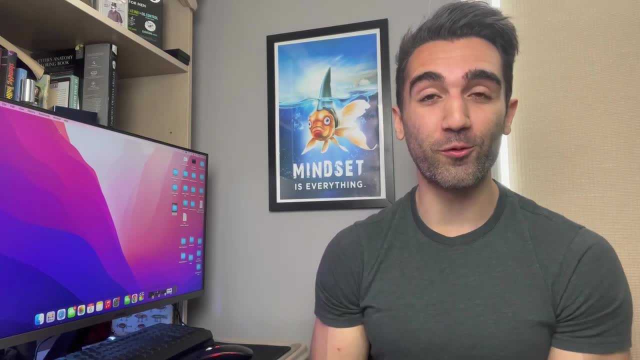 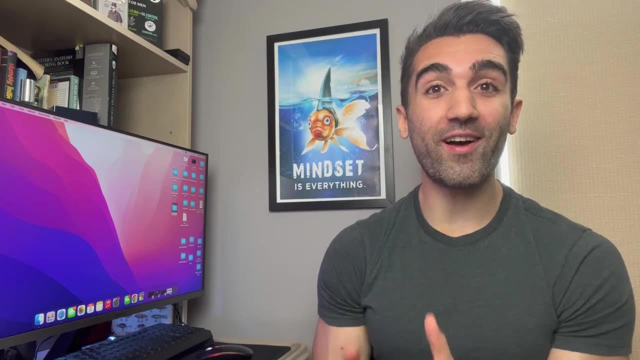 where, depending on where you would like to work, there aren't many jobs available for you. Orthopedic surgery has gained some notoriety in the last few years for individuals coming out of residency and not being able to find stable, consistent OR time and, as a result, have to resort to locums or working at different hospitals or a few different things. It is not guaranteed here in Canada that you will find a full time practice to be a part of directly after residency. Now I don't know what that process is like down in the States. 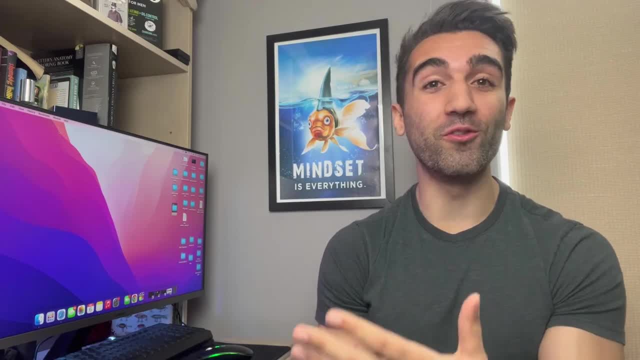 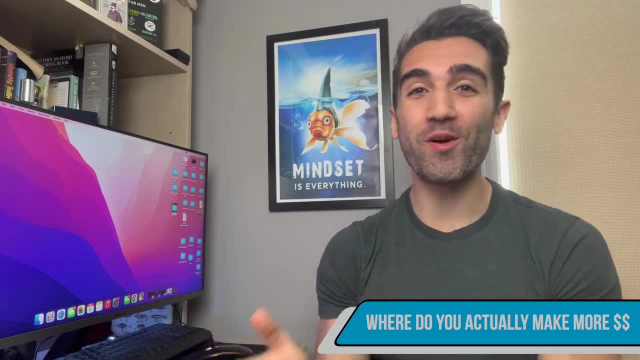 Just I thought that would be an interesting piece of information to share with anyone that was looking to get into that profession. So now, where do we stand after this entire video has done? I presented all the information to you in the original question. Do you make more money in the States or in Canada as a doctor? If you're a surgeon, definitely down in the States. I'm pretty sure the evidence will support- And then my anecdotal evidence will also support- that the surgeons down in the States tend to make a little bit more money than they do here in Canada. 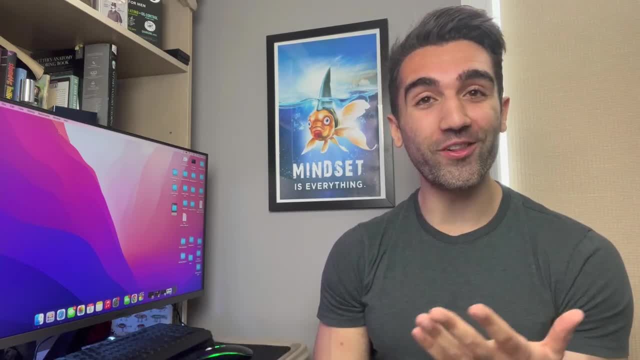 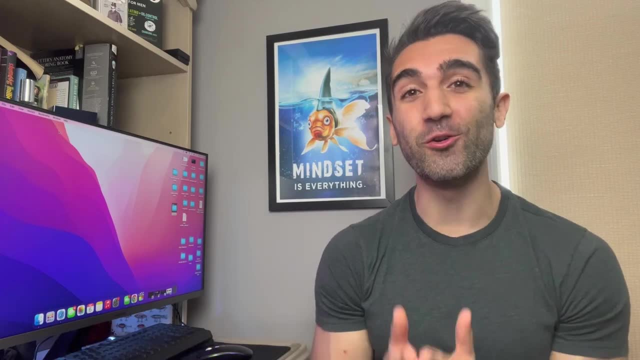 But for the rest of the specialties, I guess your mileage really is going to vary depending on the state you're practicing in, or the province you're practicing in, or also what profession, what specialty you're getting into. These are all going to be choices that you get to decide for yourself. 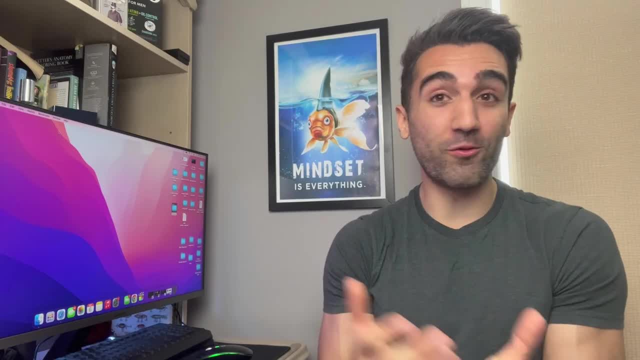 Where do you want to practice? Why do you want to practice there? You know, if you come work in Canada, for example, it might be a little bit easier in some aspects, but then you have to get through very, very cold and long winters.